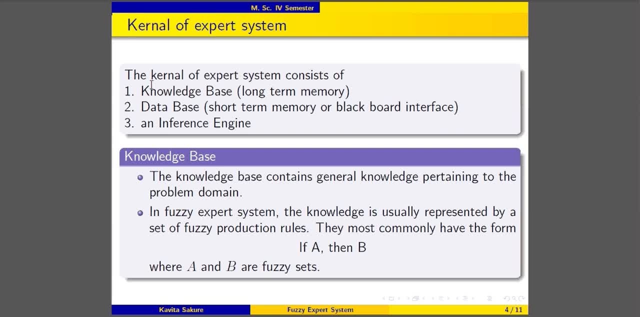 Kernel of expert system is made up of knowledge base, data base and inference engine. So knowledge base is called long term memory and data base is called short term memory or blackboard interface. So first of all we will see what is knowledge base. 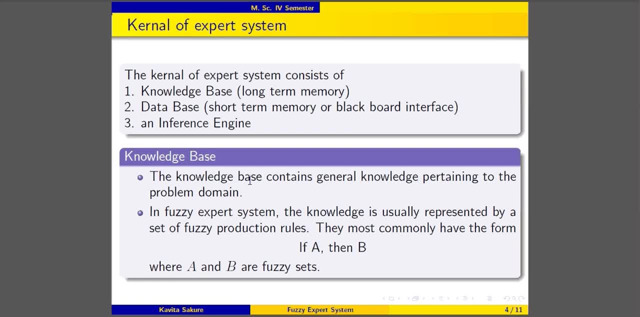 The knowledge base contains general knowledge pertaining to the problem domain Means it keeps the knowledge related to the problem domain. In the expert system, the knowledge is usually represented by a set of fuzzy production rules. Knowledge in the fuzzy expert system is in the form of a set of fuzzy production rules. 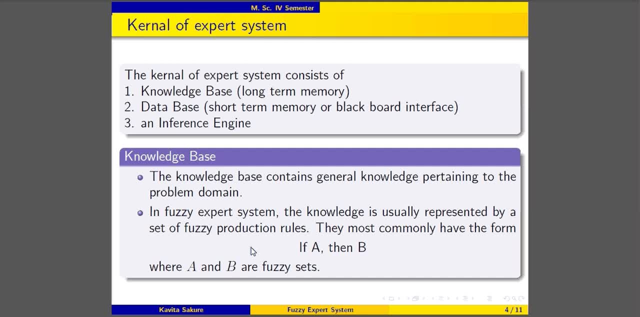 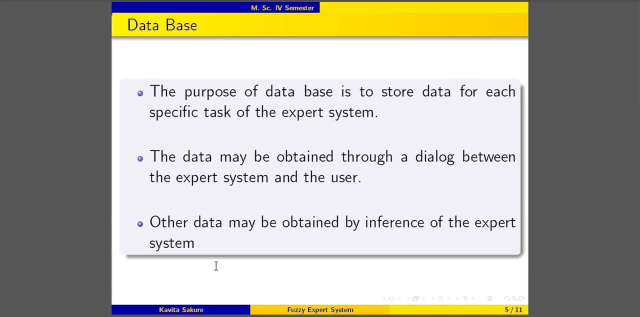 They commonly have the form if A, then B, And here both A and B are the set of fuzzy production rules Database. The purpose of database is to store data for each specific task of the expert system. The primary task or purpose of the database is to store data for any specific task. 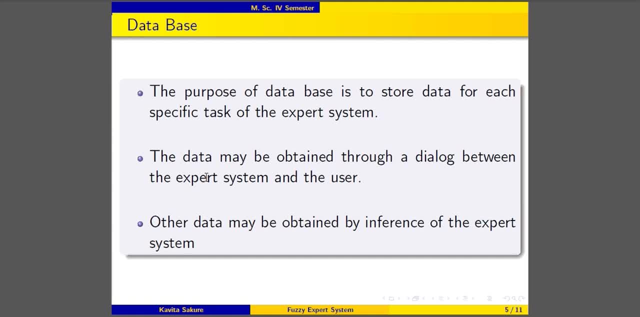 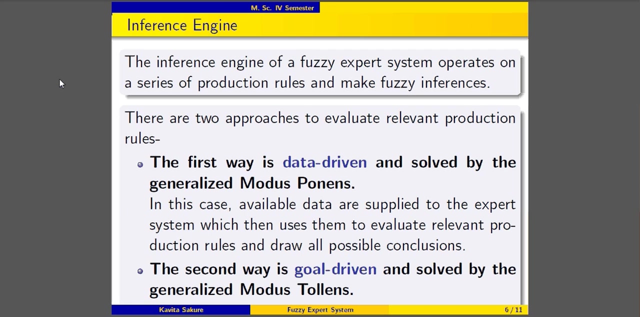 The data may be obtained through the database. Data may be obtained through a dialogue between expert system and user. Other data may be obtained by inference of expert system Inference engine. The inference engine of a fuzzy expert system operates on a series of production rules and makes fuzzy inferences. 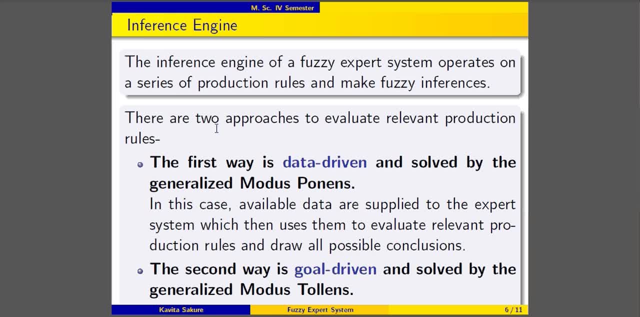 There are two approaches to evaluate relevant production rule. First way is data-driven and solved by generalized model phonemes. In this case, available data are supplied to the expert system, which then uses them to evaluate relevant production rule and draw all possible conclusions. The second way is goal-driven. 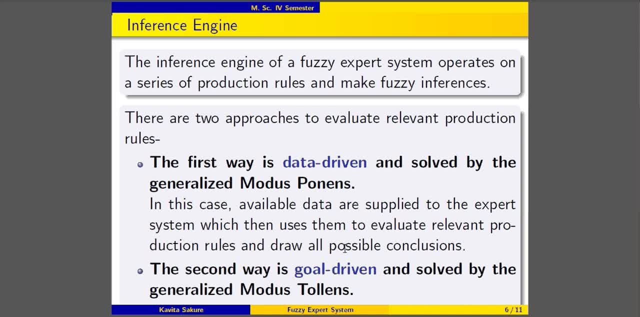 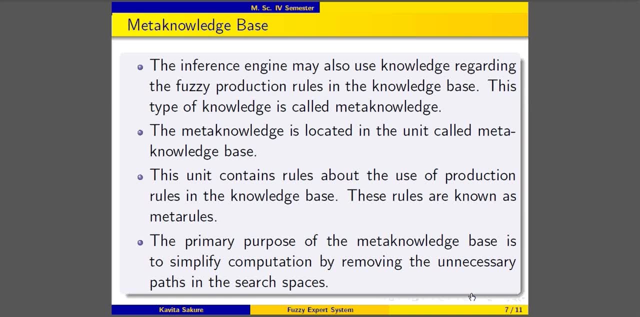 Second approach is generalised model phonemes. Third approach used in analysis is called goal-driven. The fourth approach is generalised model phonemes and the fifth approach is goal-driven. So in that case we will solve generalised models from tolerance. 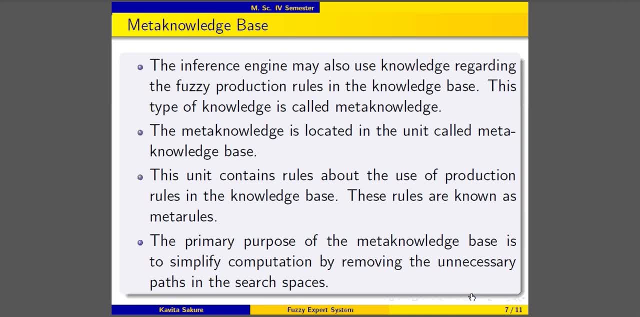 The next part of fuzzy expert system is meta-knowledge-based. The inference engine may also use knowledge regarding fuzzy production rule in knowledge based. This type of knowledge is called meta-knowledge. In this approach, primaveral knowledge or meta-knowledge is used in inference based. 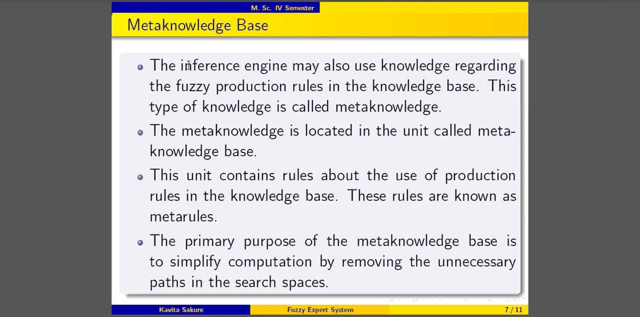 This type of knowledge is called meta-knowledge. In inference, the experimental, experimental and practical knowledge is used in analysis. In this, all the knowledge that is going to be used in the production rule is called Meta-Knowledge, and Meta-Knowledge is located in the unit called Meta-Knowledge Base. 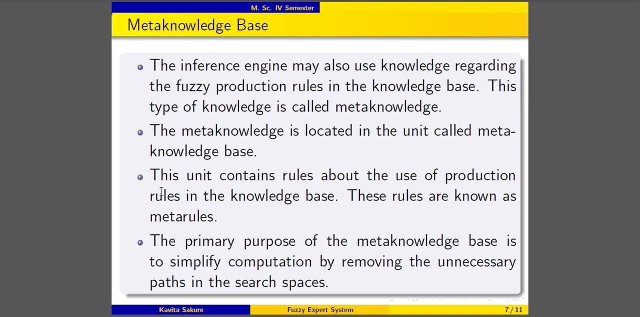 Meta-Knowledge will be contained in Meta-Knowledge Base. The unit contains rules about the use of production rule in knowledge base. These rules are known as Meta-Rules. The primary purpose of Meta-Knowledge Base is to simplify computation by removing the unnecessary paths in such spaces. 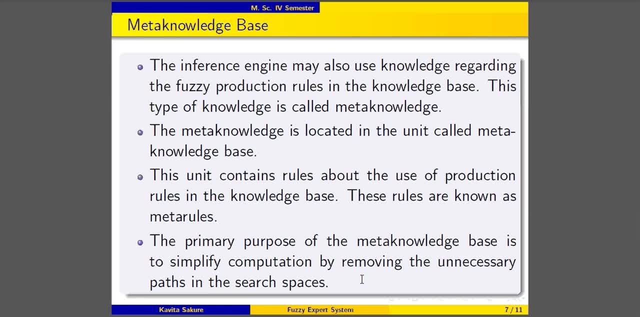 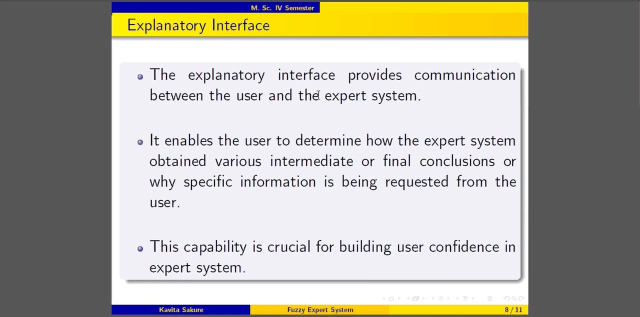 The primary purpose of Meta-Knowledge Base is to immediately use the data and knowledge that we need. This is the main purpose of Meta-Knowledge Base Explanatory Interface. The explanatory interface provides communication between user and expert system. It enables the user to determine how the expert system obtains various intermediate or final conclusions and why specific information is being requested from the user.